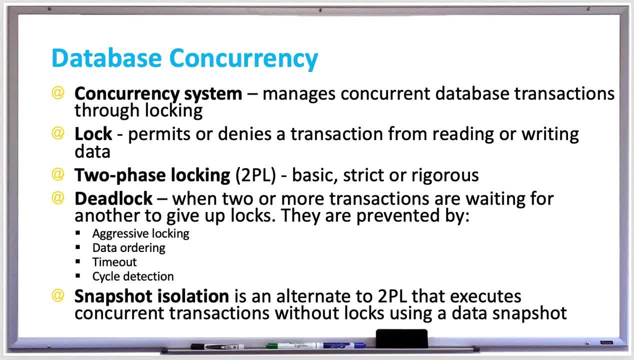 Lock scope could also be a block or the whole table. in the case of where a transaction needs to access several rows of data, A lock scope could also include indexes. The concurrency system figures out when to grant or release locks by monitoring active transactions. Lock requests. 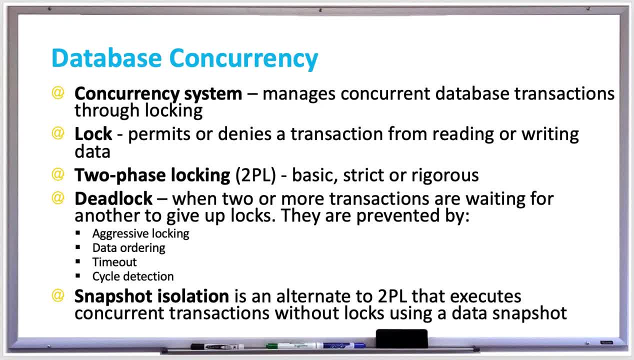 are handled by the lock, The lock manager, which tracks, grants and releases locks. The concurrency system implements each transaction's isolation levels by requesting shared and exclusive locks as needed, And the concurrency system also reduces the duration of transactions that are waiting for lock data. 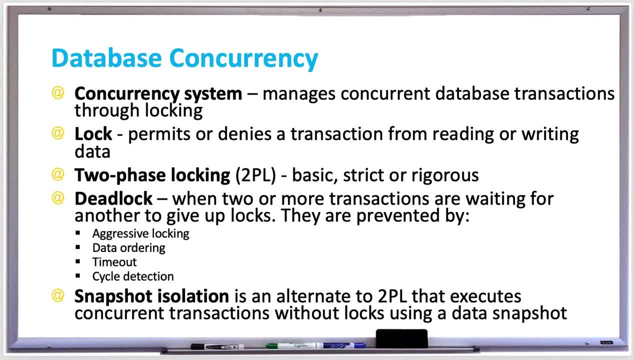 by minimizing lock scope. So 2PL stands for two-phase locking, which is basic, strict or rigorous. A serializable isolation level means that a transaction is independent from other transactions. So a lock is a lock manager which tracks, grants and releases locks. The concurrency system implements each 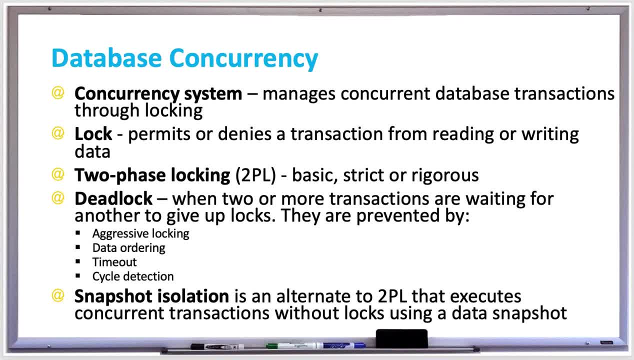 other transactions, And there's three types of two-phase locking which help prevent conflicts and ensure serializable transactions. There's basic two-phase locking, where a transaction is set to follow the basic two-phase locking protocol And if locking and unlocking can be done in just 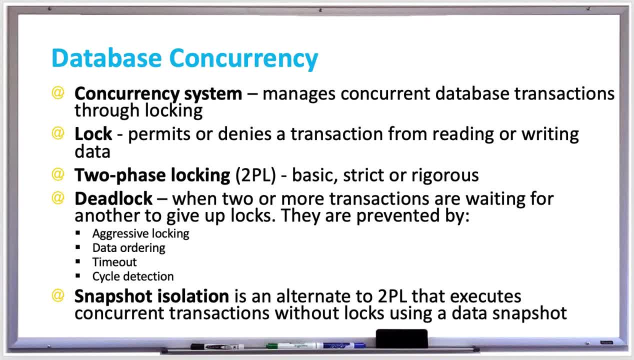 two phases, which are the growing phase or shrinking phase. Growing phase is where new locks on data items may be acquired, but none can be released, And shrinking phase is when existing locks may be released, but no new locks can be acquired. Strict two-phase locking is when 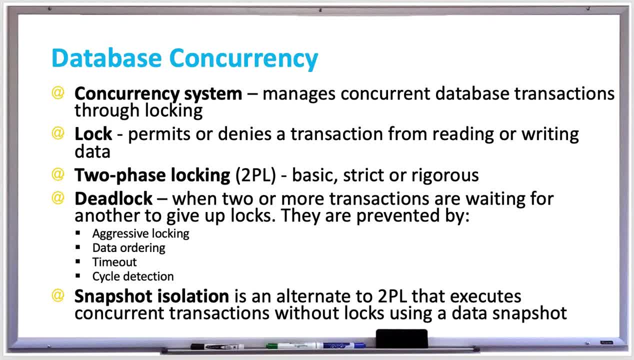 a transaction must hold all its exclusive locks until it commits or aborts, And most relational database concurrency systems implement this type. There's also rigorous two-phase locking, where a transaction holds both shared and exclusive locks until the transaction commits or rolls back, And this type is easier to implement than strict but not as efficient. 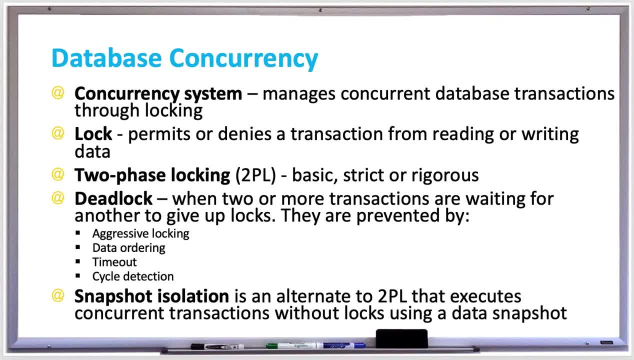 because shared locks are held longer. A deadlock is a situation in which two or more transactions are waiting for another to give up locks. A dependent transaction is waiting for data locked by another transaction And a cycle of dependent transactions indicates deadlock has occurred. Concurrency systems manage and prevent deadlocks in several ways. They use aggressive 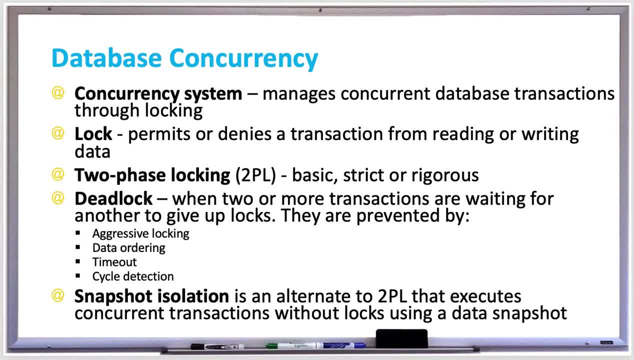 locking. It's where each transaction starts with a request to all locks, And if all the locks are granted, then the transaction runs to completion, And if not, the transaction waits until all other transactions release the locks. Then there's data ordering And the data. 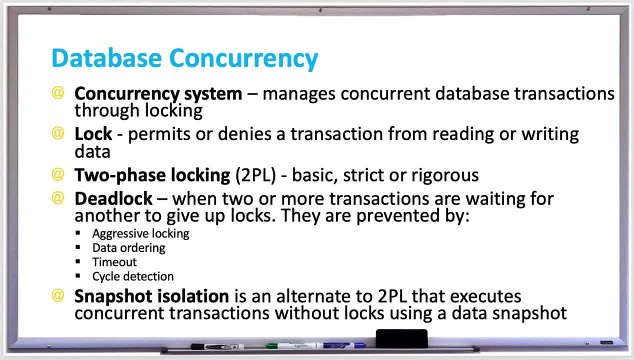 is ordered and each concurrent transaction takes locks in order. There's timeout, where each transaction requests the lock rolls back if the lock's waiting exceeds a fixed period of time set by the DBA. And cycle detection, where, if the concurrency system discovers a cycle of dependent 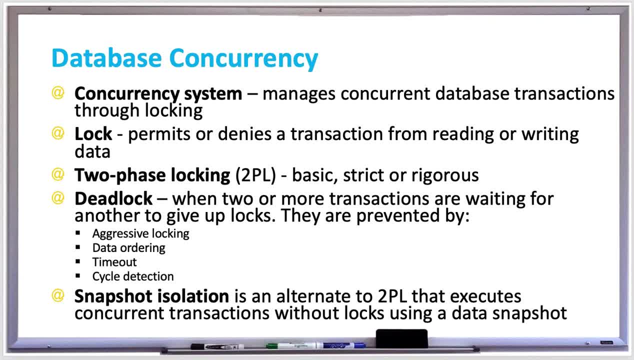 transactions. then it selects and rolls back the locks, And then there's timeout, where each transaction checks the lock. So at least one transaction will be locked. Let's move on to Snapshot isolation. Snapshot isolation is a popular alternative to 2-phase. 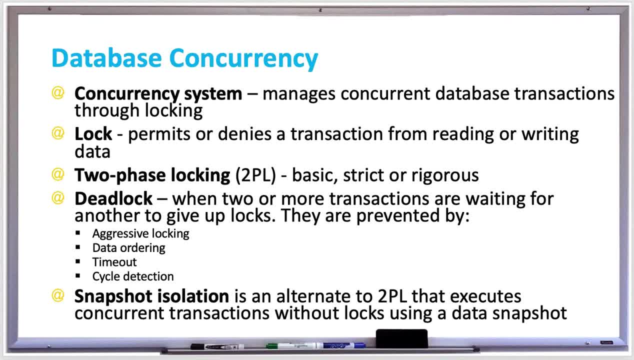 locking. Snapshot isolation is an optimistic technique which executes concurrent transactions without locks by creating a snapshot of the data. so the transactions never wait but may sometimes restart if all of the operations are processed, the data that's read or written by the transaction, and then it writes updates to private copies of. 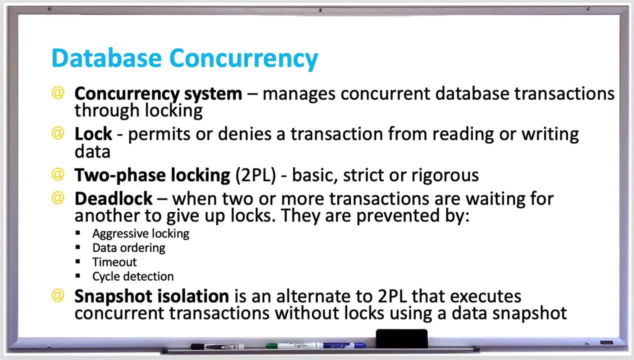 the data, Then it determines if there's any transaction conflicts with an update and then it writes updates to the database or just rolls back the transaction. And there's also a serializable snapshot isolation, which is a serializable version of a snapshot isolation. 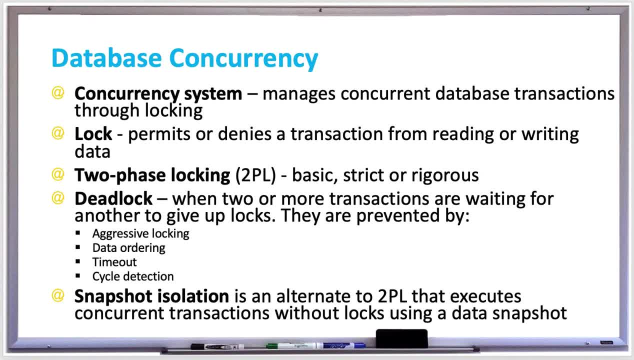 which ensures serializable schedules when isolation level is set to serializable. Thank you.